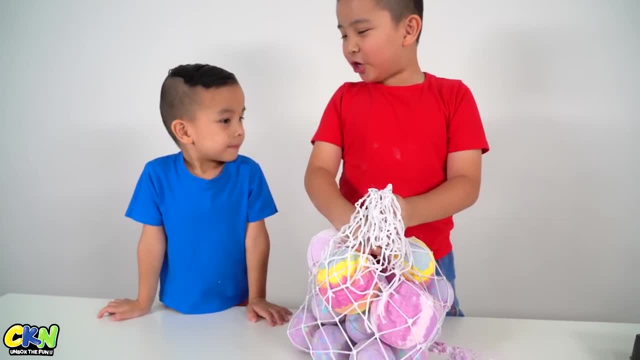 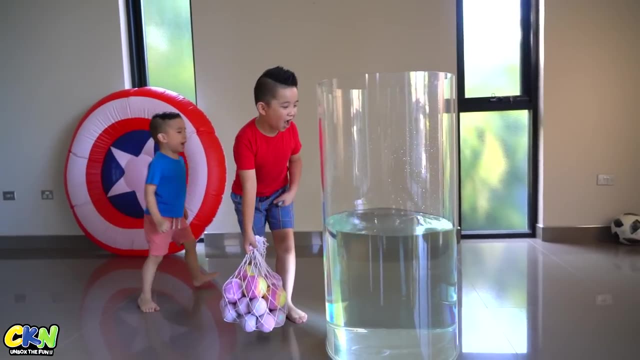 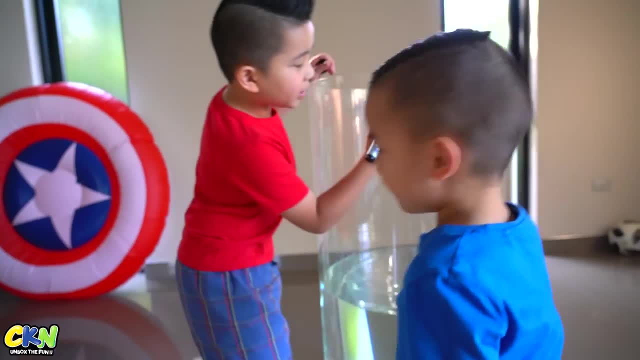 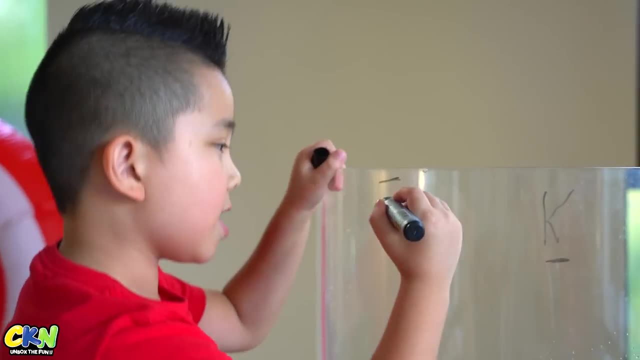 Yeah, All right, Kyson. where do you think it'll go up to There? Okay, Now, I think it's going to be all the way up to here. Oops, All right, Are you ready, Kyson? Yeah? 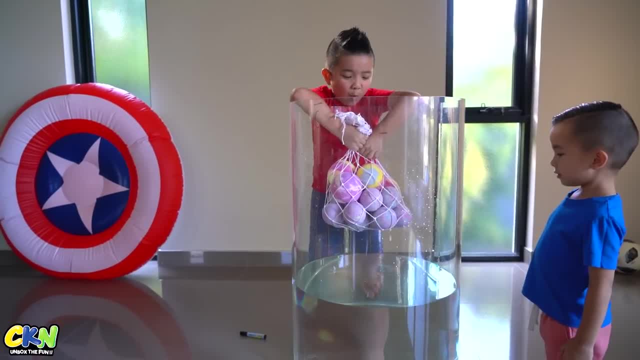 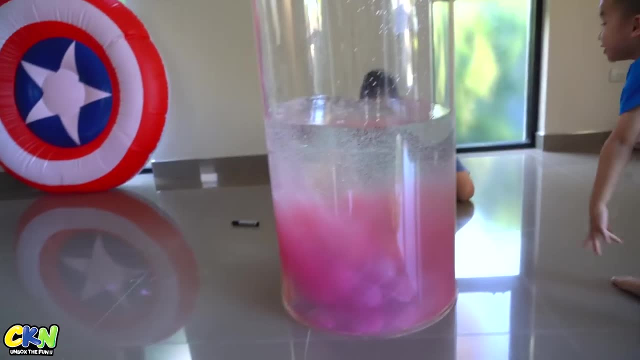 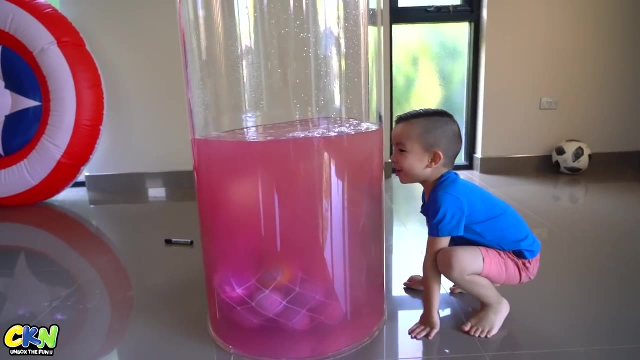 Three, two, one. Ooh, Whoa, Whoa, Whoa, Whoa, Whoa, Whoa. Oh, smell it. Wait, I want to smell it too. Wow, look at the color. It smells so nice. 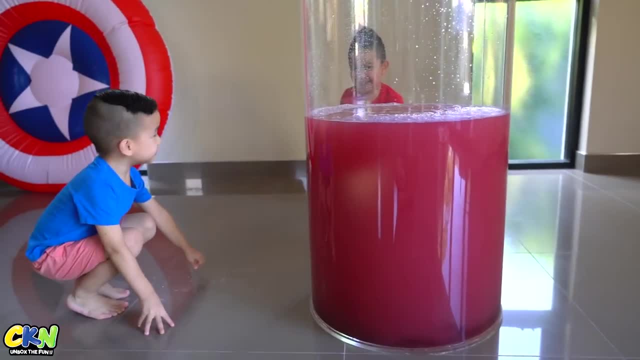 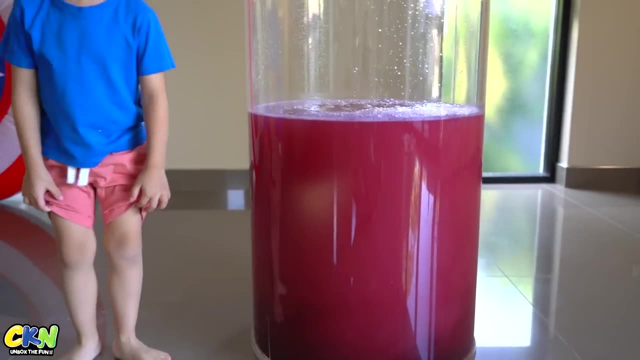 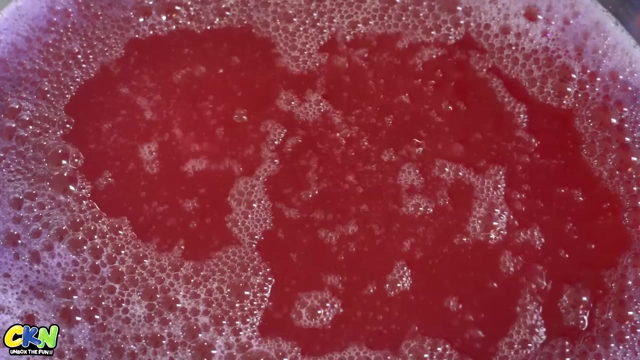 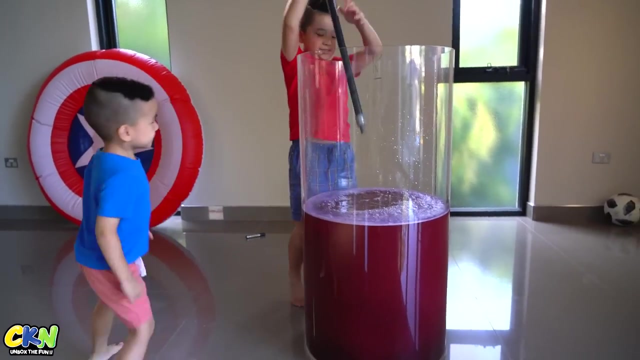 I can smell it. Wow, Look at the color. It smells like gum Here. look Gum. It's at the bottom. It looks like a throat. Alright, Carlton, I'm going to mix it. It's like purple on top. 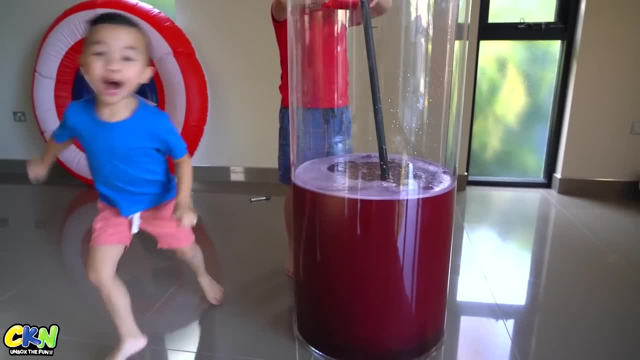 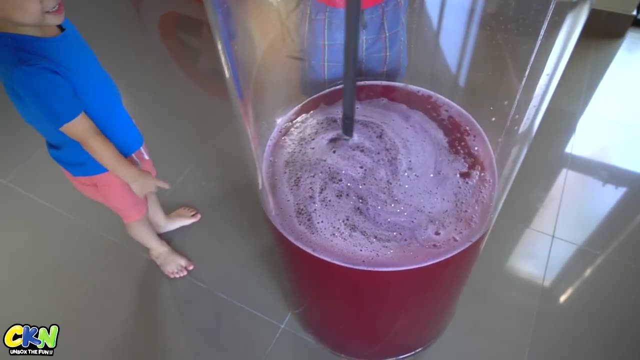 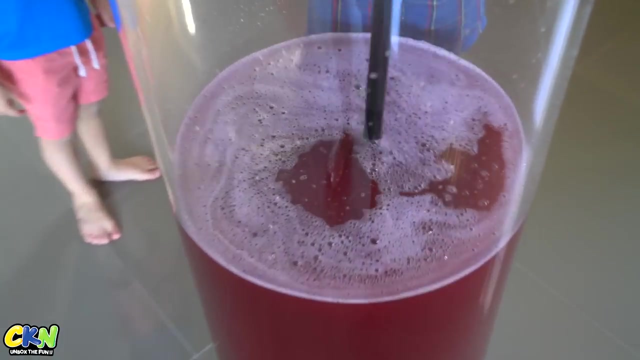 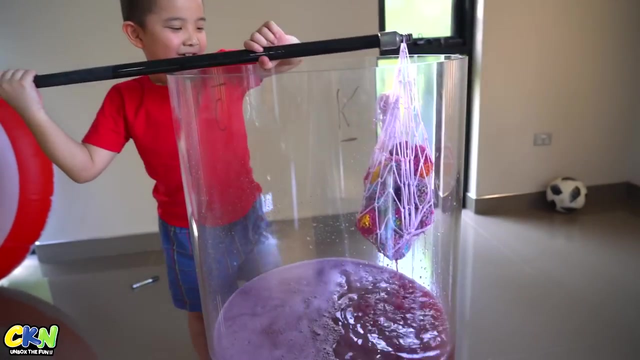 No, it's not purple on top. Look at the bubbles. You're playing catch. You're playing catch with the bubbles. Look how many bubbles there are. Get all the bubbles. Look around. What is this? It looks like something from the sea. 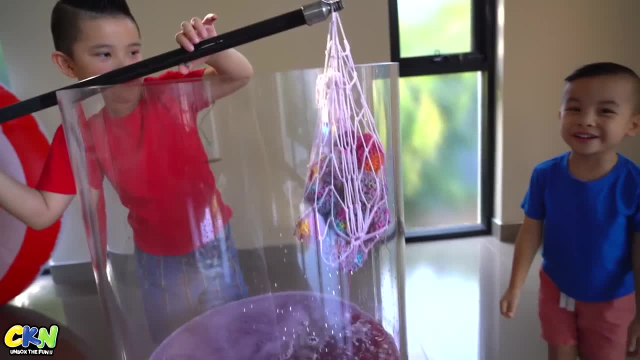 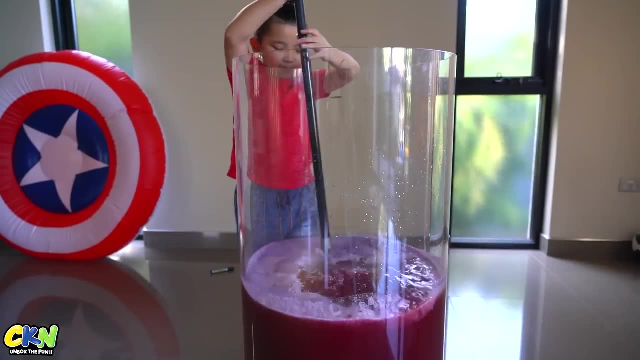 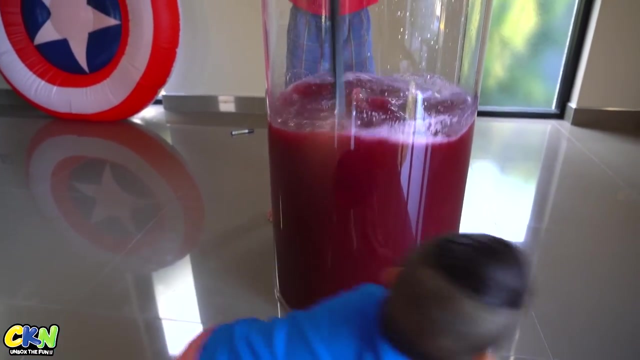 Carl or something. Oh, I just touched something. Do you think we should drop it inside here? Yes, Wow, Let's see what it is. I know where it is. Oh, no, No, it's not there. I don't know where it is. 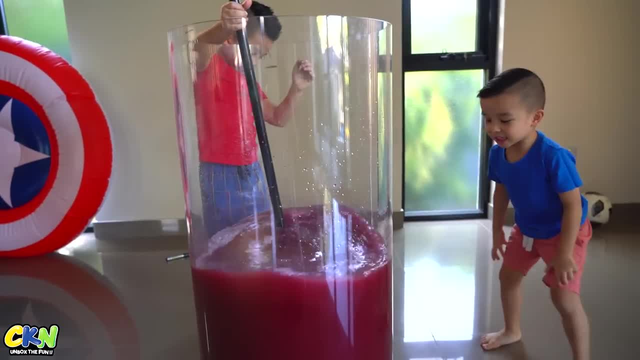 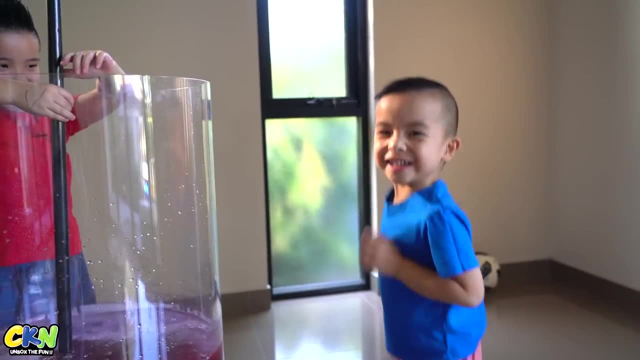 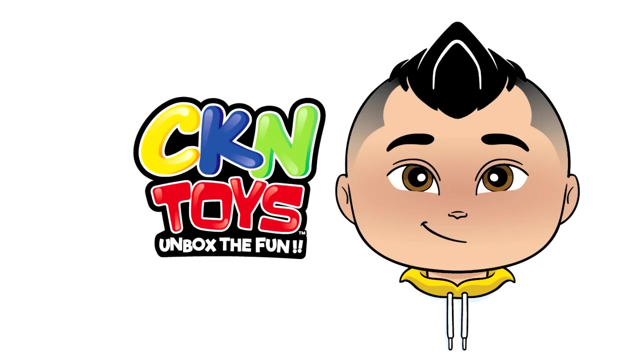 Stop it, Look, Keep mixing it so I can look at it. Alright, let's see who the winner is. Carlton- Yay, So I get to get the Carlton. What Huh?